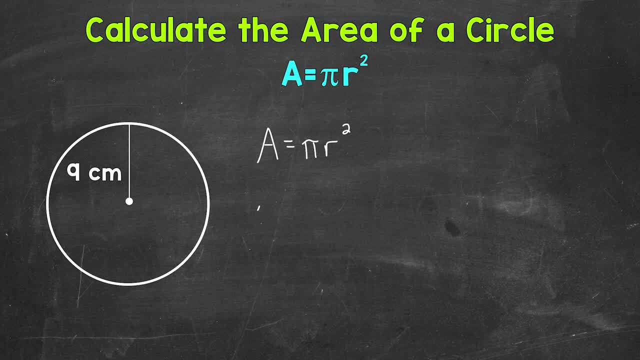 Then I'm going to plug in the radius. So area equals Pi times the radius, which is 9 centimeters squared. After that let's do 9 squared, which means 9 times 9, not 9 times 2.. 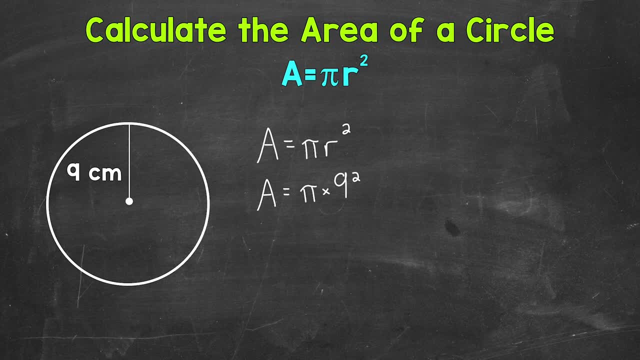 That's a common mistake. So remember 9 squared: when you square a number, that means multiply that number by itself. So 9 squared means 9 times 9, which is 81. So we end up with pi times. 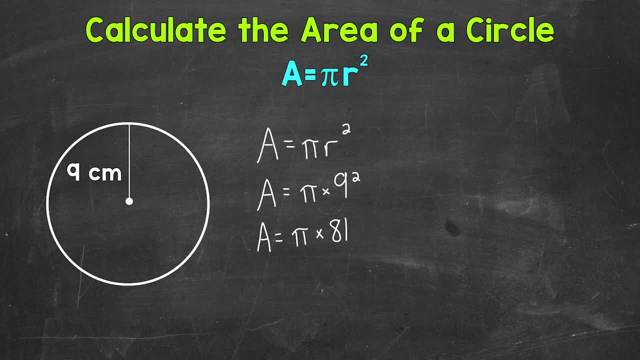 81. Now we can rewrite this as: area equals 81 pi. One way to write the area of a circle is to write it in terms of pi Meaning. we can write our number in front of the pi symbol and put our unit of measure, which is centimeters. 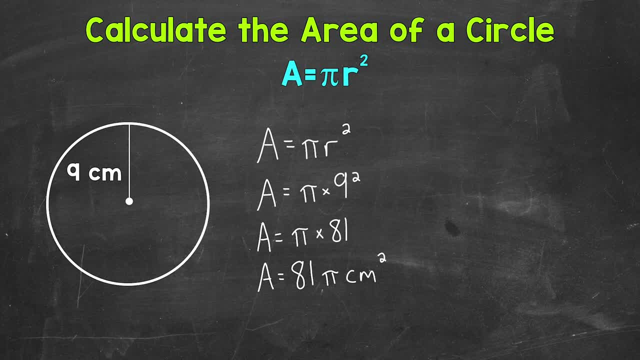 And when working with area, it's going to be squared. So we have area equals 81 pi squared centimeters. So again, one way to write our answer is in terms of pi. So we have our number and then our pi symbol, followed by the unit of measure squared. 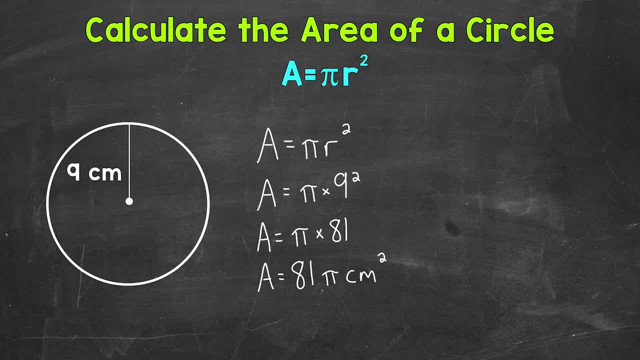 Now another way we can do this is to use an approximate version of pi. Like I mentioned earlier, we're going to use 3.14. So pi is approximate, Approximately 3.14.. So that squiggly equal sign there. that means an approximate value. 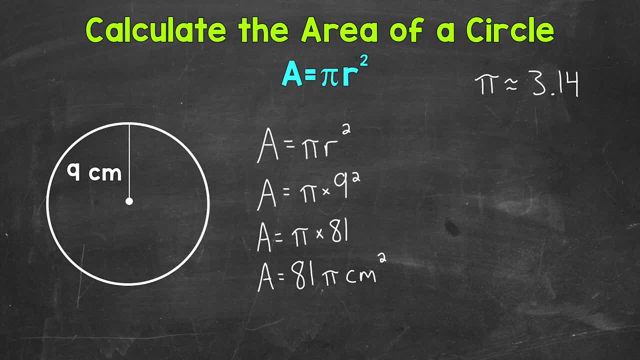 Unlike an equal sign, which means an exact value. So something to keep in mind when you see that. So let's go through our process here, And we're going to start by writing out our formula. So area equals pi r squared. Next let's plug everything in. 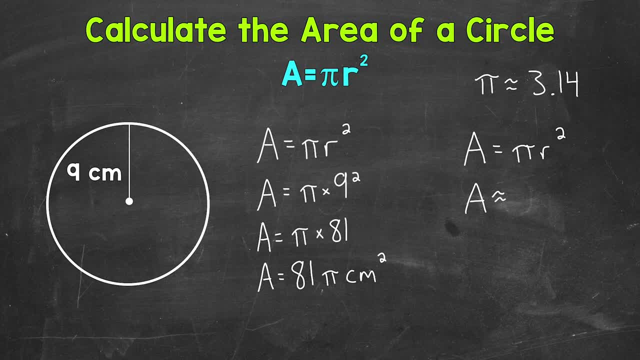 So we have area. Area is approximately- and I'm using the approximately symbol since we are using an approximate version of pi. So 3.14 that we're using for pi times our radius of 9 centimeters squared. So 9 squared is going to give us: well, we have 3.14, and 9 squared equals 81..